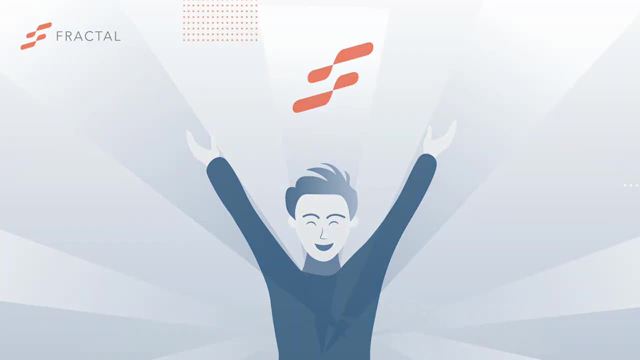 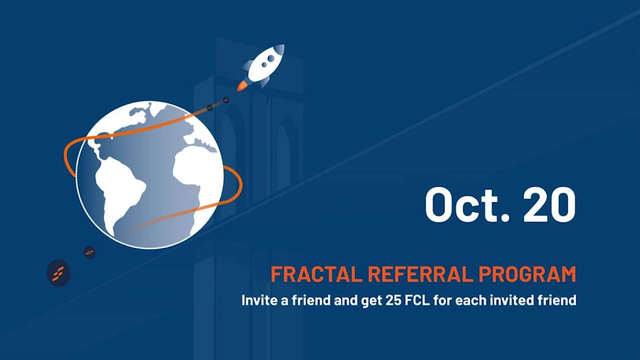 This video will be about Fractal's vision for a new data economy, a demonstration of Fractal's product, the Fractal ID wallet and, last but not least, you'll get some information about Fractal's upcoming referral program. Let's begin with Fractal's vision. Fractal's vision is to 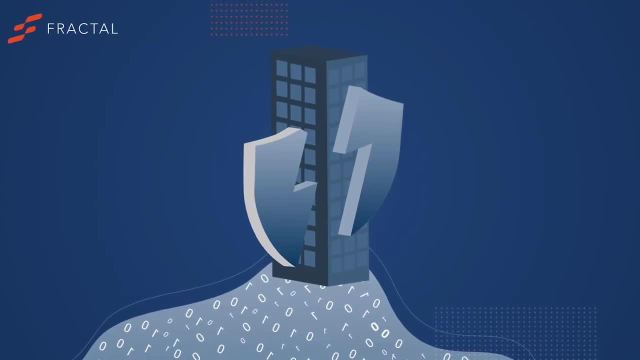 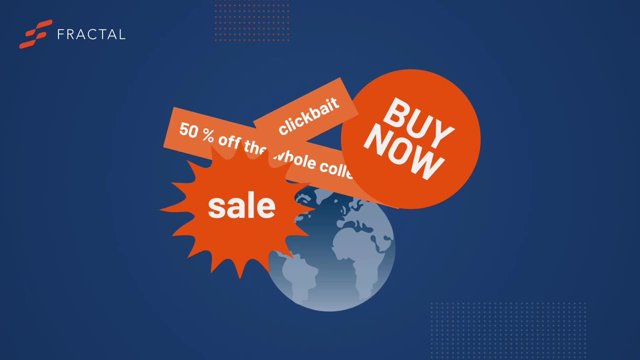 create an open and fair data economy. The current data economy has been pretty much the same for over 30 years, where the web has been using online advertising as the most viable monetization strategy for content creators and publishers. Online advertising therefore remains the prime. 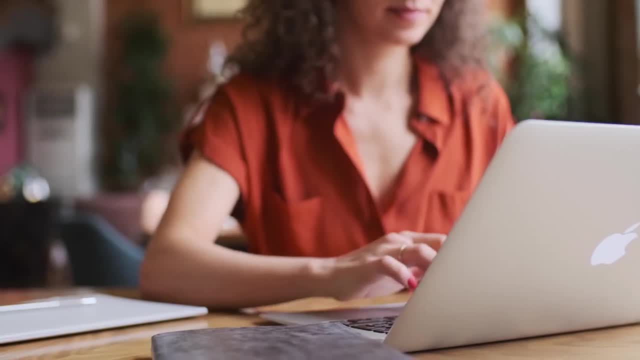 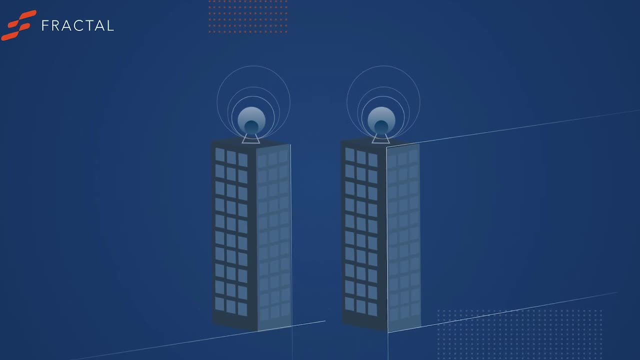 source of funding for most content on the web. The ad market relies on the accurate targeting of potential consumers browsing the web. However, data is often collected from users browsing the web without their consent or their knowledge. The majority of collected data on users are: 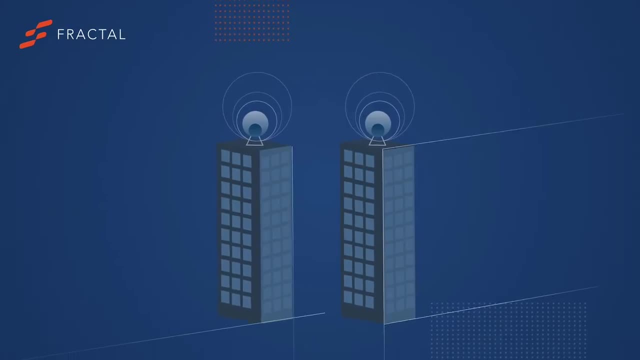 performed by two well-known tech giants. These companies make up a duopoly in the ad market, which creates a non-competitive market where no stakeholder benefits from the dropouts. These companies likely take advantage of the different speed and prioritization of the market, reducing the overhead to just a few other influencers. In fact, they don't actually. 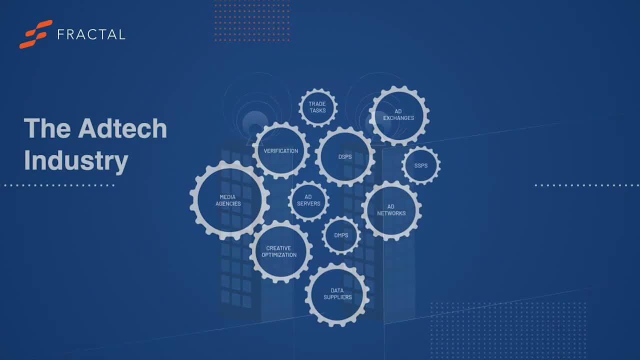 droppalistic structure, except for the droppalists themselves. The ad market itself is also heavily inefficient for advertisers because of the complexity of the ad market infrastructure and fraud. About 56% of digital ad spend is served to the wrong audience, never actually displayed. 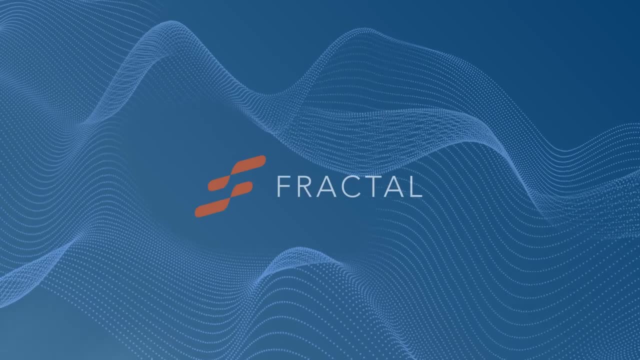 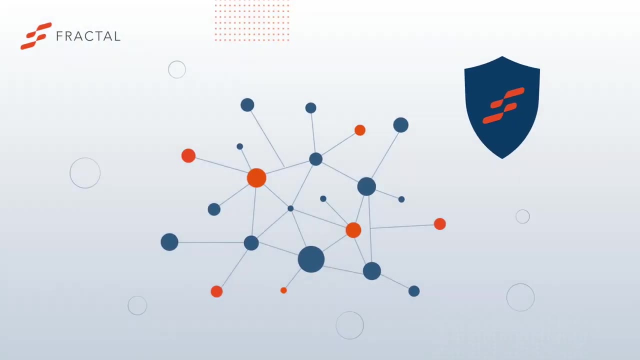 or consumed by bots instead of humans. These are a few of the issues with the current data economy that Fractal have a vision and a solution for with their new data economy To achieve a new and improved equilibrium within the ad market infrastructure where all stakeholders benefit. 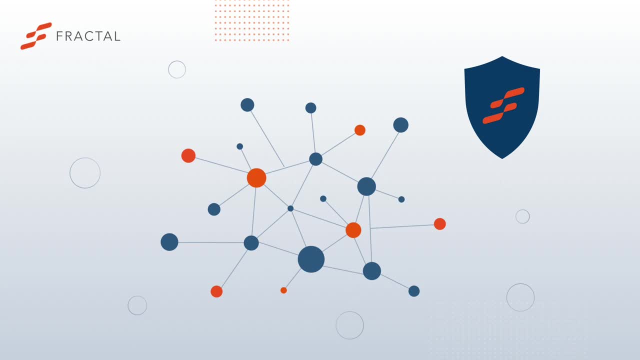 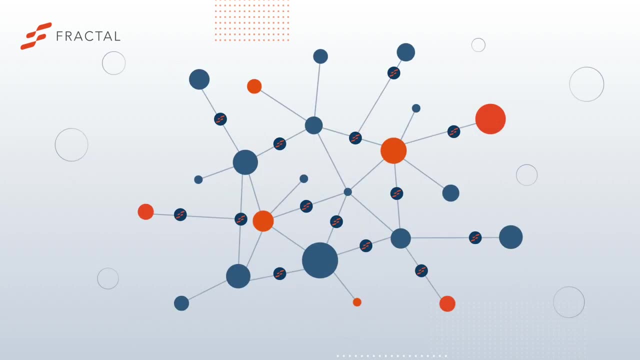 Fractal proposes an incentive system for the sale and purchase of data built on a transparent, privacy-preserving and trustless infrastructure. This incentive system is enforced through the use of blockchain technology, delivering verifiable guarantees of said enforcement and a trustless public record, allowing stakeholders to monitor each other's behavior in a privacy-preserving 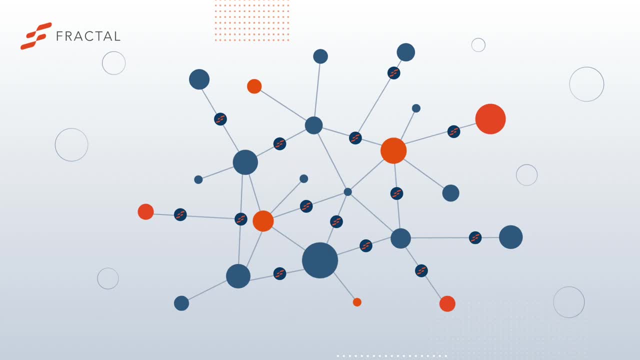 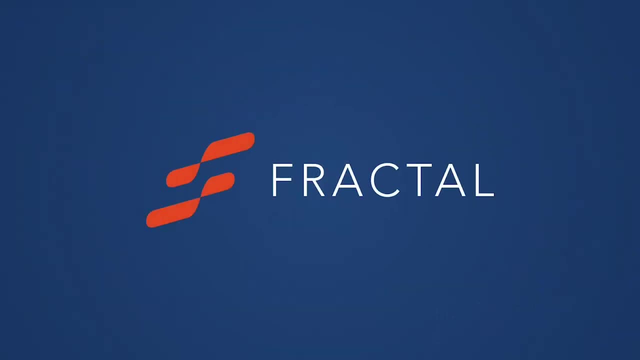 manner. This will also, in itself, function as a disincentive to fraud. So what does Fractal do? What does it mean for the users? In status quo, your data is taken, used and sold by somebody else. With the Fractal protocol, this changes. In short, users will be able to use applications like the: 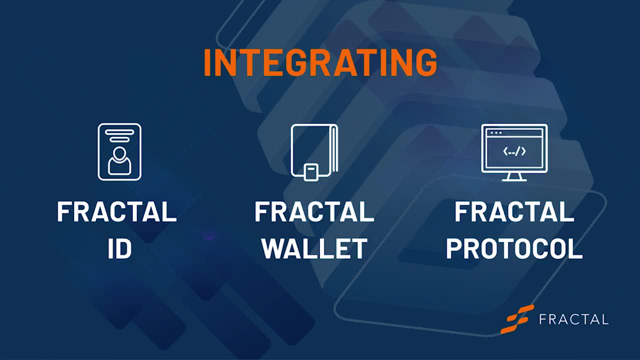 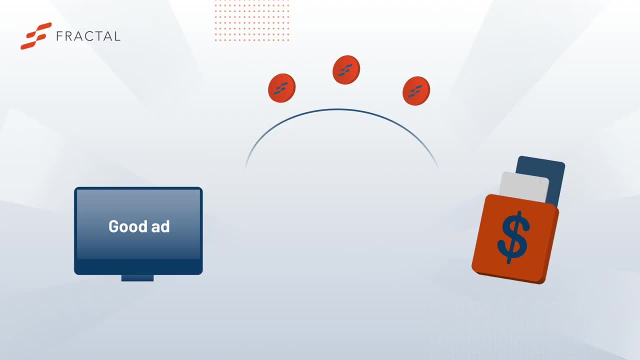 Fractal ID wallet that is built on top of the protocol's technical infrastructure, which empowers the users to control and own their data. It provides the opportunity for every user to get fairly compensated for sharing one's own data with sites and services that the user has previously. 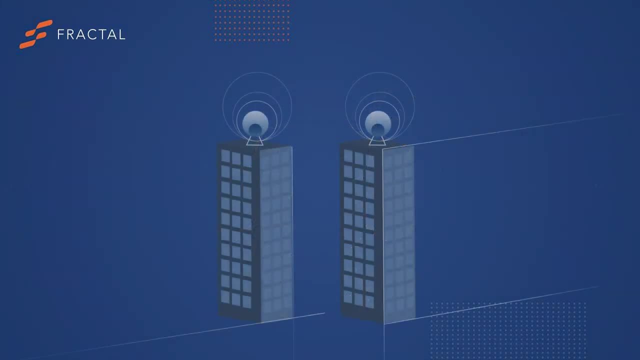 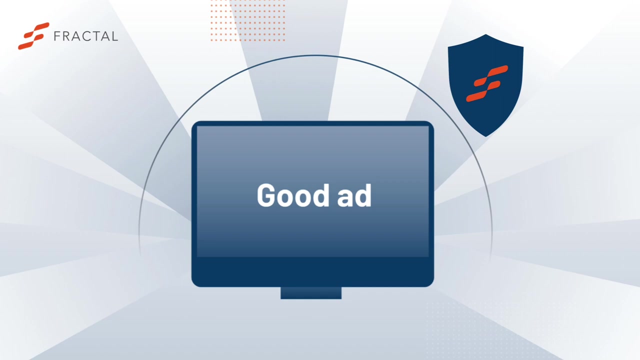 defined. What does this mean for the ad market? Well, the billions of dollars that are spent on duopolic inefficiencies, as well as data fraud, can be meaningfully invested in ads. that leads to real, genuine traffic with real results Everyone. 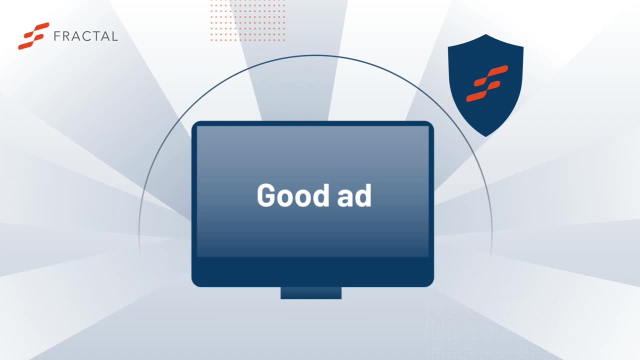 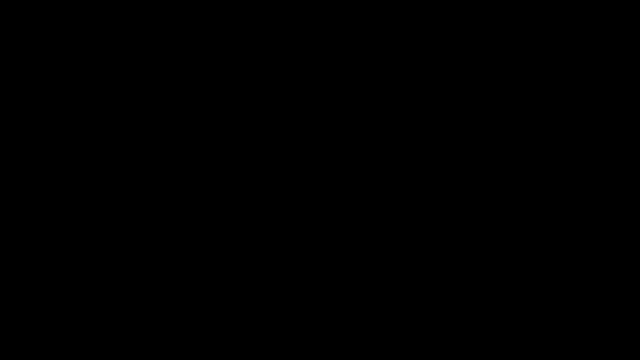 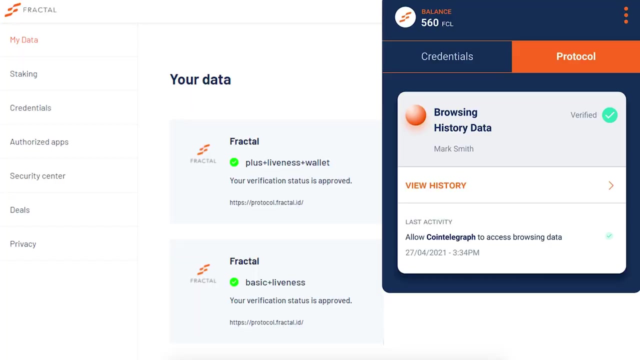 the content publishers, the ad tech companies and the advertisers profit from such a revolution- Everyone, except for the two giant companies that have controlled the industry for far too long. Now we move on to the Fractal ID wallet demonstration. The Fractal ID wallet is a decentralized identity wallet built on top of the protocol's technical infrastructure. This is a decentralized identity wallet built on top of the protocol's technical infrastructure. The Fractal ID wallet is a decentralized identity wallet built on top of the protocol's technical infrastructure. This is a centralized identity wallet built on top of the protocol's technical infrastructure. 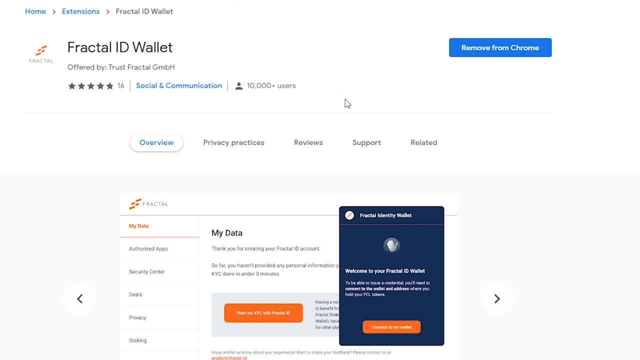 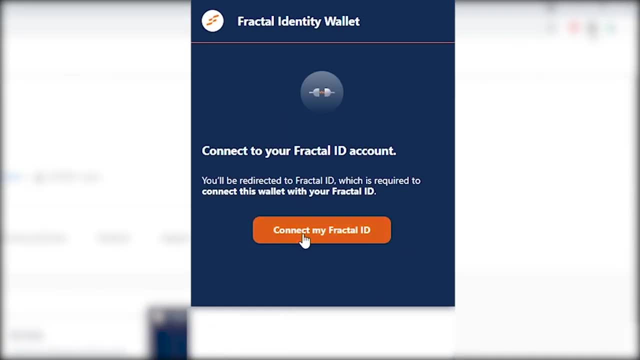 that simply works as an extension on the google chrome browser. simply download the wallet from the chrome webstore. when you open the extension, you'll create your own password and then be directed to fractal id, where you will create an account. verify your id and login. once you have logged in, click the. 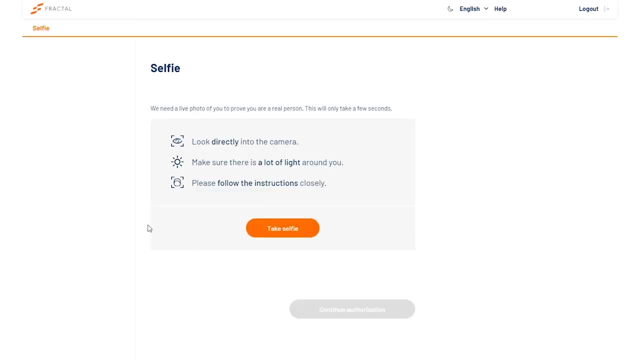 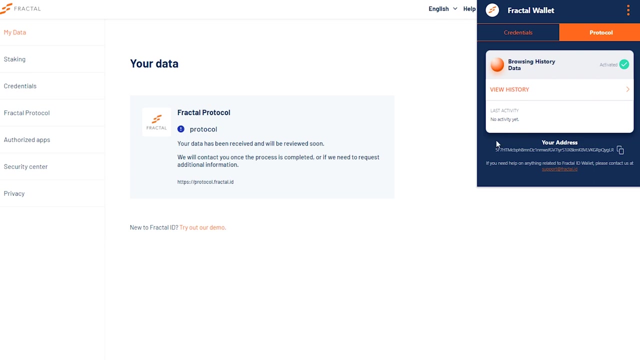 buttons saying join the fractal protocol. submit the selfie as a liveness check and it will say: your data will be reviewed shortly. in the meantime, open the fractal id wallet extension again: click, click. join the protocol, click create and continue. There you will see your very 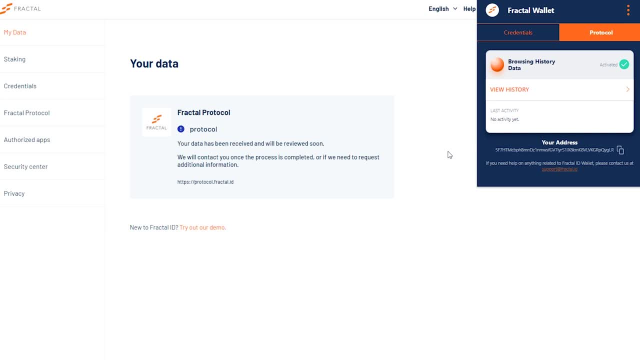 own FCL token address, And you are now done. Now, when you browse around the web, the Fractal ID wallet will safely store your browsing history in your device and reward you with FCL tokens for your data, And that's it. There are already more. 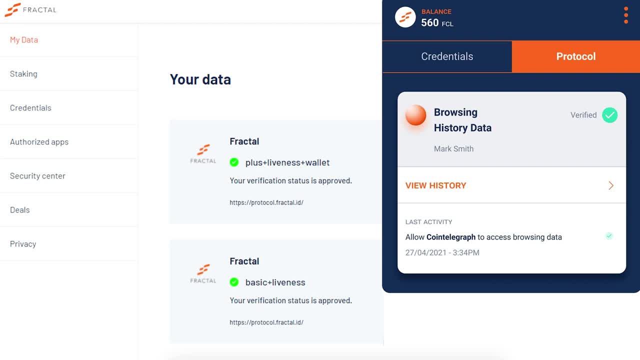 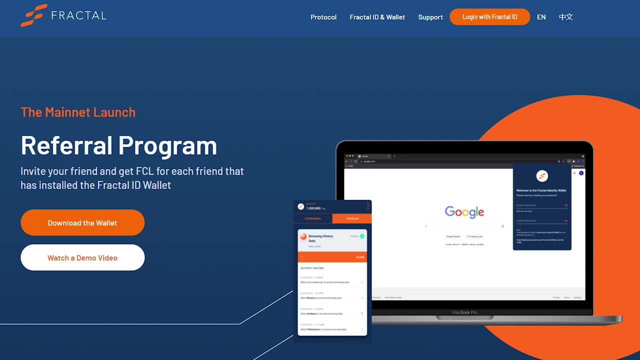 than 10,000 users using the Fractal ID wallet and have been doing so successfully since the testnet launch. And now you will as well. And now we move on to the last part, an explanation of Fractal's upcoming referral program. 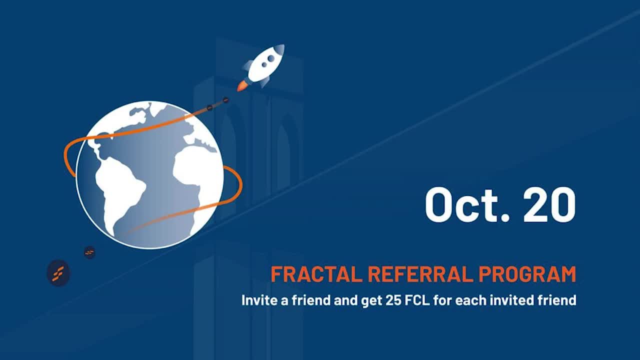 To celebrate the upcoming mainnet launch on the 19th of October, Fractal will initiate the referral program on the 20th of October, which lets anyone invite their friends to download and use the Fractal ID wallet in exchange for referral rewards. If the invited friends installs the Fractal wallet, both you and 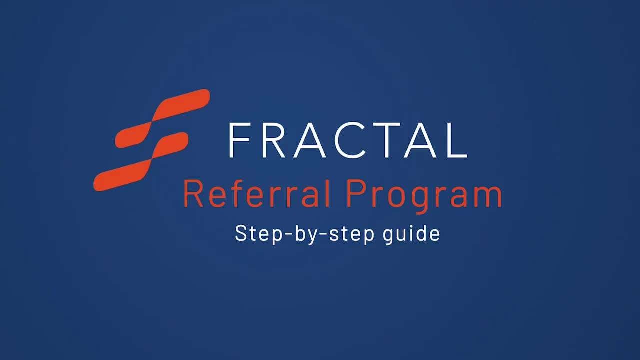 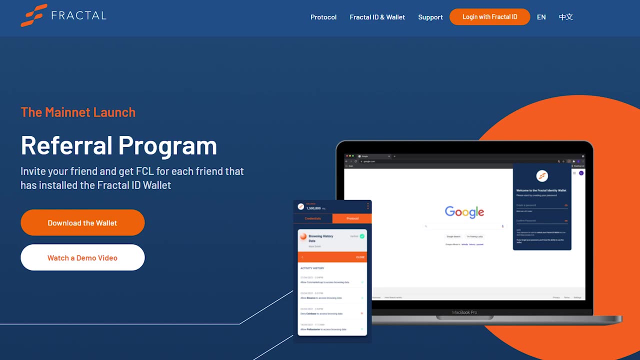 your friend will get 25 FCL tokens. What follows is a step-by-step guide on how to participate in the referral program. All steps regarding the referral process are managed on this page. Let's first take a look at how to invite friends On the page. you'll see a referral pop-up here in. 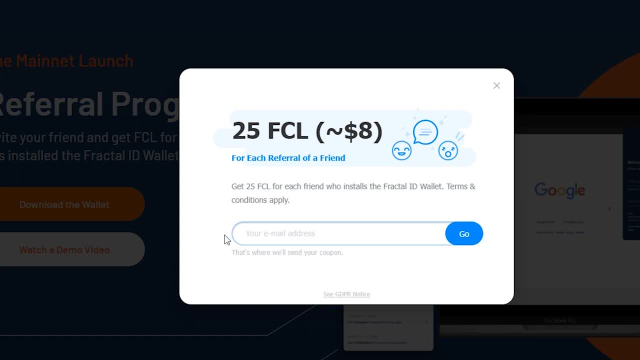 the upper right corner, which you'll need to fill out to participate. After giving your mail address, the system will generate a unique link for you with which you can invite your friends. But wait, that's not all. To claim your award for inviting friends, you also need to have the wallet installed and set up. 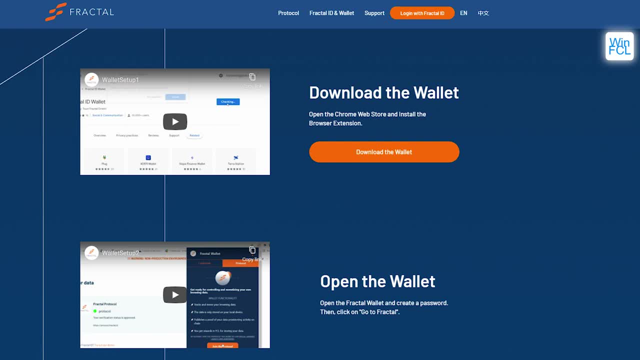 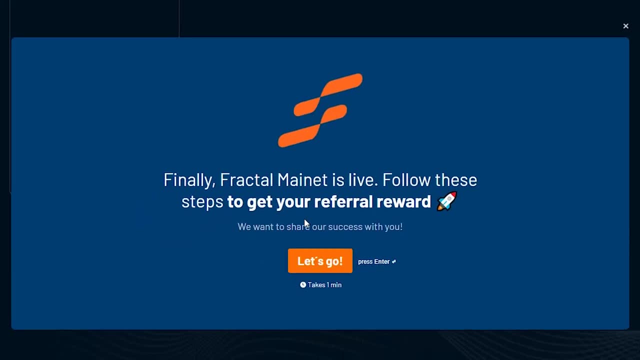 yourself. If that's not the case, follow the instructions on the page to do so. In the final and last step, you will need to download and use the Fractal ID wallet to fill out the type form. This is super crucial, because here you will be asked to. 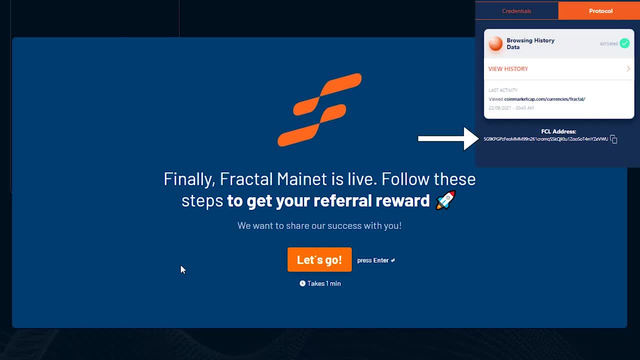 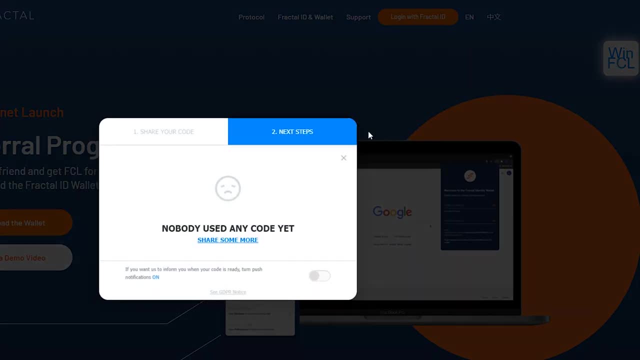 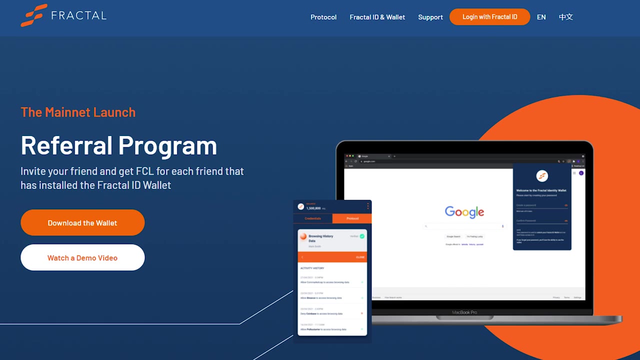 insert your mail address and your address from the Fractal wallet, which is the destination to which your rewards will be sent. After all of this have been done, you can now go ahead and invite all your friends with your unique link. You can always find your unique link here in the upper right corner. Now let's say you: 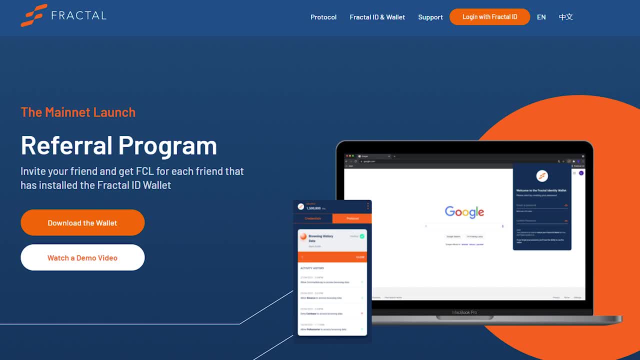 have been invited and you want to claim your reward For this. you need to click on the unique link from your friend. The link will be in the upper right corner. The link will direct you to this referral campaign page. Here you will also see a. 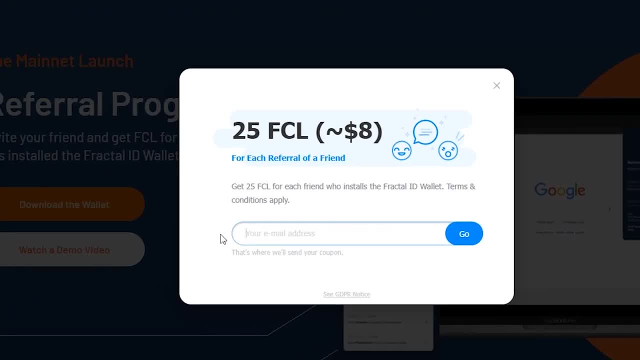 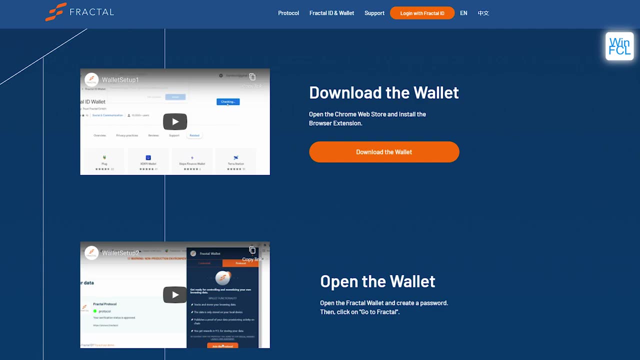 popup. Fill it out with your mail address to confirm that you have been invited by the friend to whom the link belongs. Then follow the instructions on the page to download and set up the fractal wallet. In the last and final step, you as well. 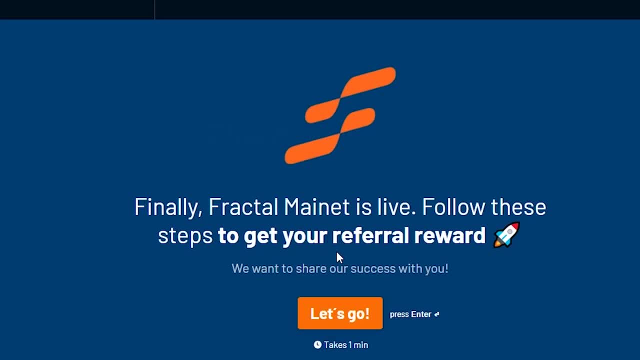 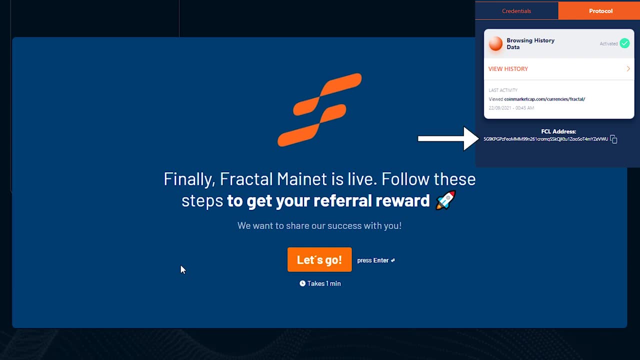 need to fill out the type form. This is very essential because here you will provide Fractal with your fractal wallet address, to which the funds will be sent. If this is done, you will become 25 FCL tokens richer. If you want to gain even. 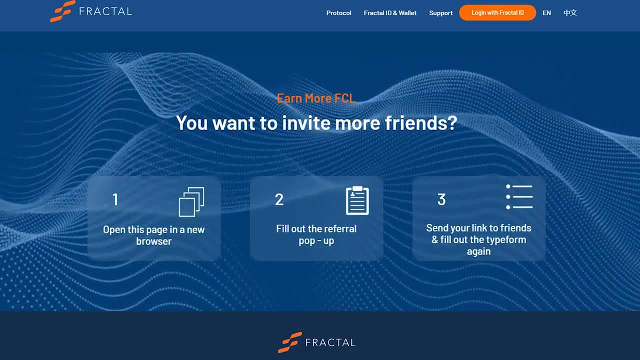 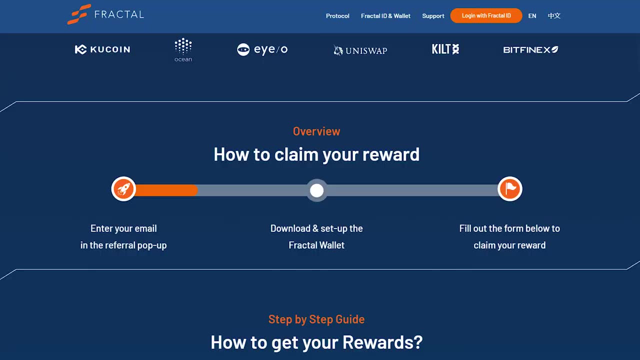 more FCL tokens. you can, of course, also invite friends yourself To do so. you need to reopen the fractal referral page in a new browser or in the private mode, Remember, in order for you and your friend to get your 25 FCL tokens each. 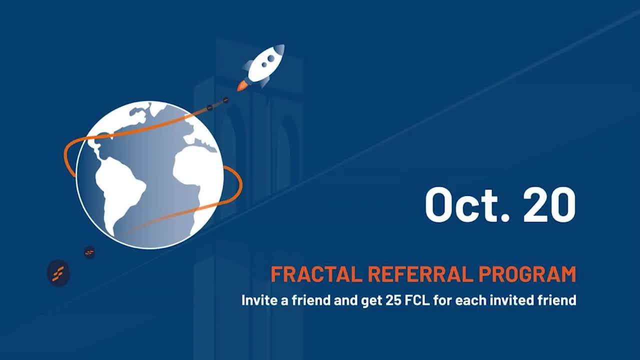 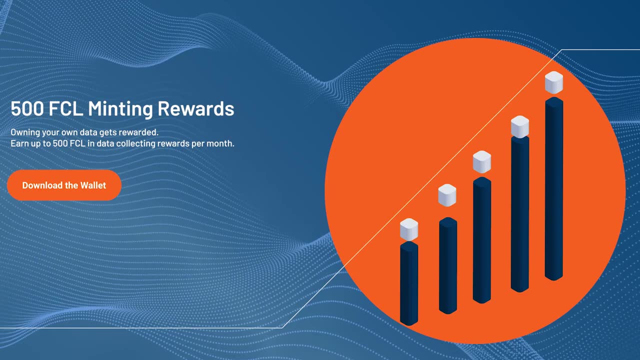 you both need to have installed the wallet. In total, you can claim 15 rewards summing up to 375 FCL tokens. And, by the way, we highly recommend not to uninstall the wallet, as you will get up to 500 FCL tokens per month by just having it.